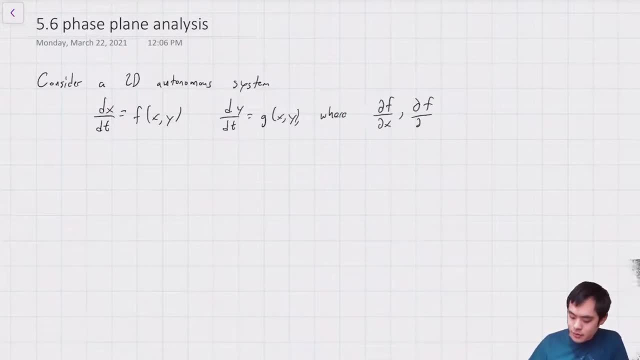 So df, dx, df, dy, dg, dx, dg, dy are continuous. Okay, so the first thing to note is by the existence uniqueness theorems, existence, uniqueness: only one solution up the translation. So only one solution passes. I can't spell passes. 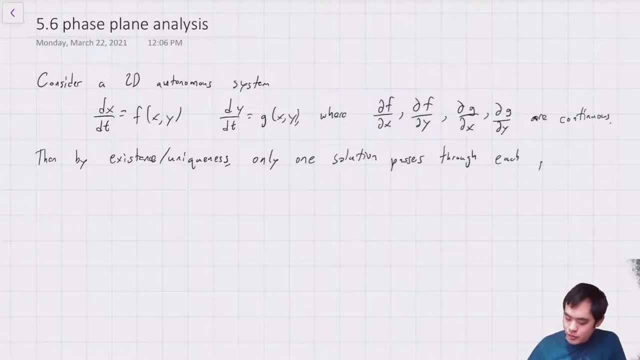 through each point in space So we can draw out vector fields. Vector fields, Yeah, In the phase plane. Okay, so let's guess There's a couple options, Option one which is just to draw out vector fields, out vector fields for every point. 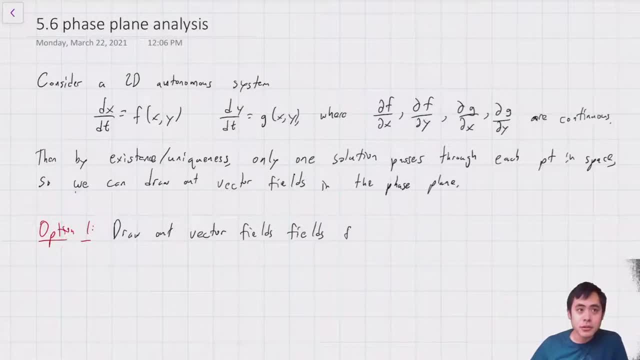 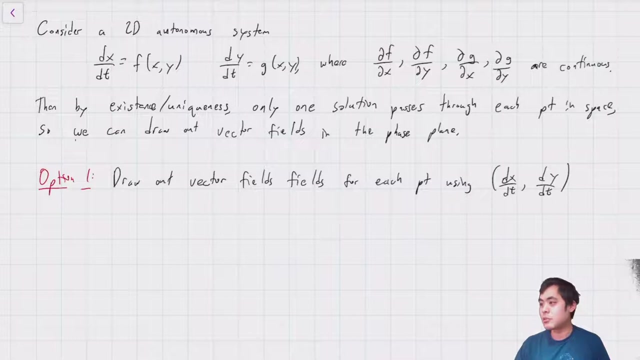 Now this is possible if you have a computer for each point. Okay, so if you have a computer for each point, Now this is possible if you have a computer, but it's a little bit more difficult if you're going to be doing it by hand. 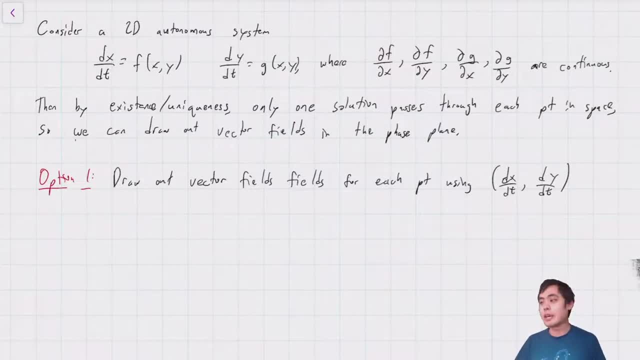 It turns out that, although you can do this by computer, sometimes it's useful to do it by hand, because with certain types of analysis, you can prove things about global stability of these systems. Option 2, which is what we're going to focus on today, is what's called nocline analysis. 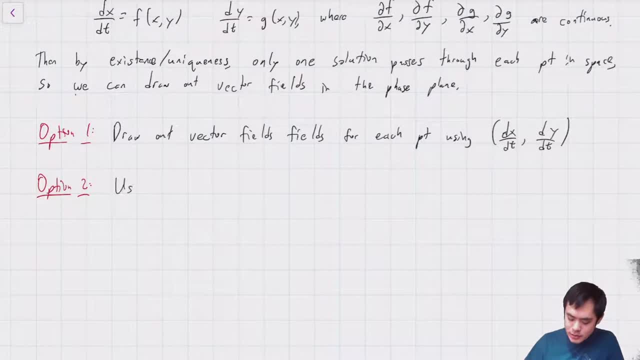 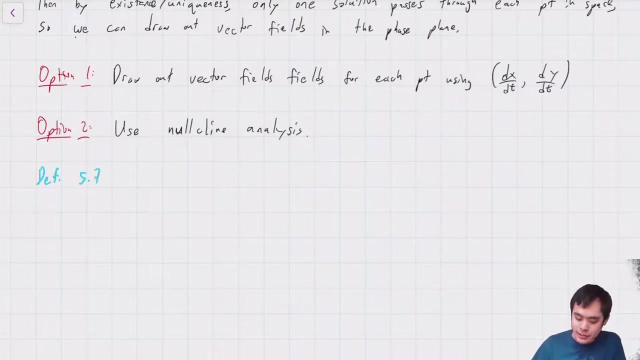 Use nocline analysis. So let's define this and then we'll give an example of how this can be applied. So this is definition 5.7 in your textbook. So the x0 isocline, also known as the x nocline. 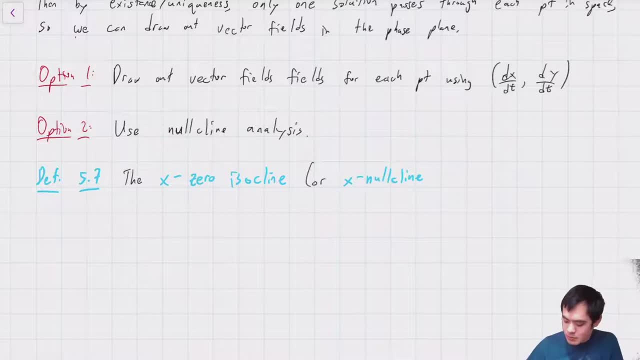 So an isocline is just a. Let me finish defining this first. So this is the set of all points, x, y satisfying f of x, y is equal to 0.. And the y0 isocline or the y nocline. 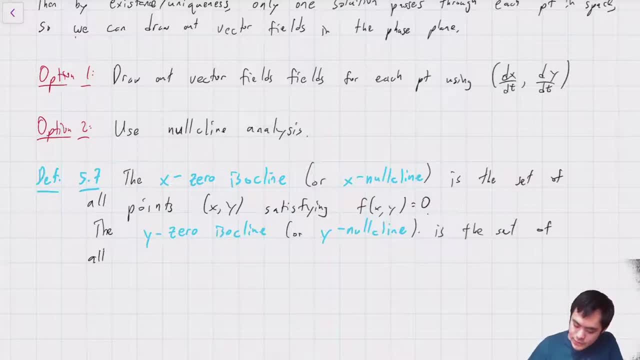 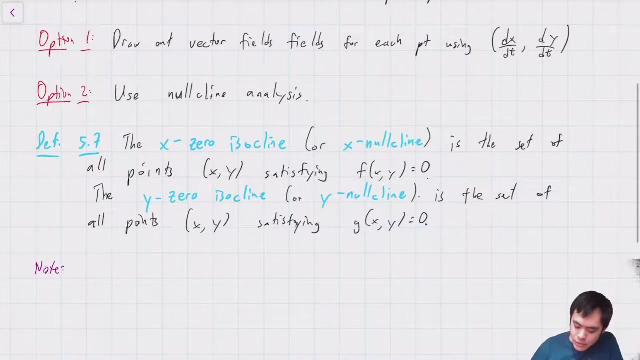 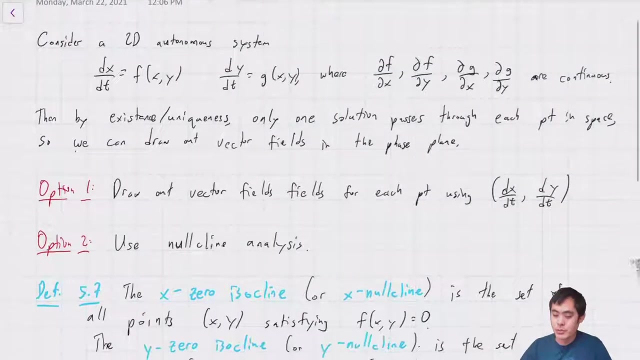 is the set of all points that satisfy g of x- y is equal to 0. So basically, what we're doing is we're solving f of x- y equals 0 and g of x- y is equal to 0 separately. So recall that when they're both equal to 0, you have an equilibrium. 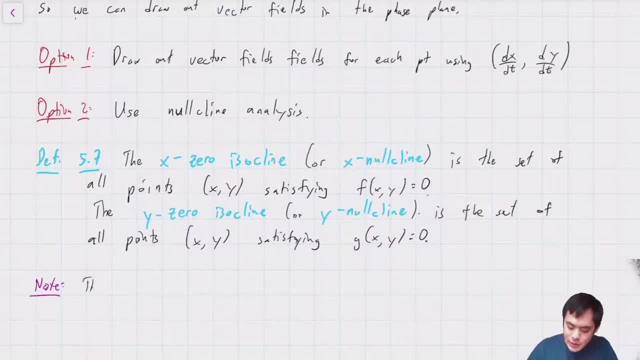 And now we're just going to solve each one separately. And it turns out that analysis has some very nice properties. So the x and y noclines intersect at the equilibriums, at the equilibria, Because that's obviously where both of them are equal to 0.. 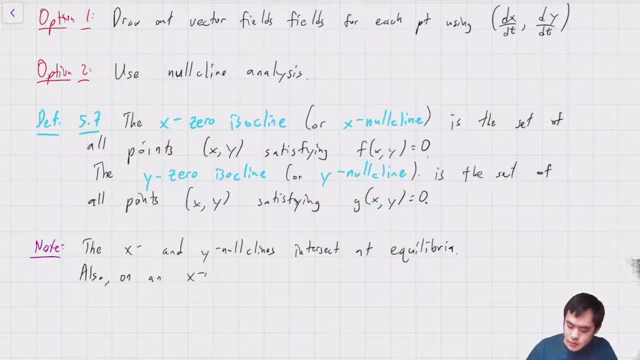 Also, on an x nocline, solutions can only move up-down, Because on an x nocline you know that the x component of the vector field is equal to 0. And so the solutions can only move up and down because those are the y components. 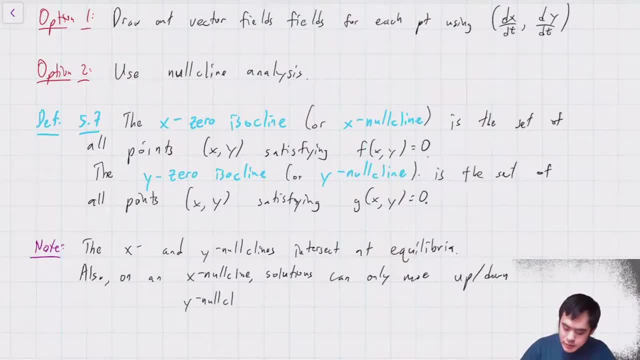 So up-down And on a y nocline solutions can only move left-right For much the same reason. Just a quick note on terminology. The reason we call this a zero isocline. so an isocline is a set where f of x, y is equal to some constant c. 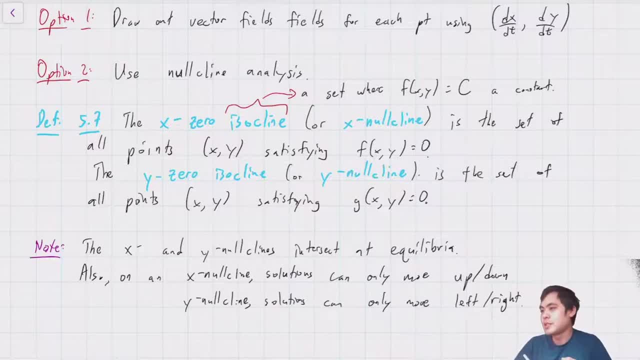 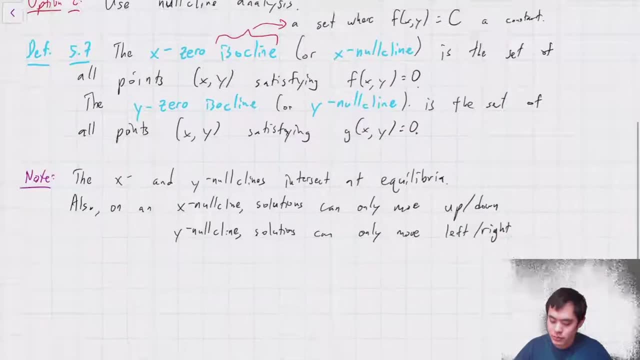 And the other isoclines are also similar, So sometimes useful in graphing these things out. But we're only going to talk about the zero isoclines, And so those are because those are so often used in this kind of analysis. 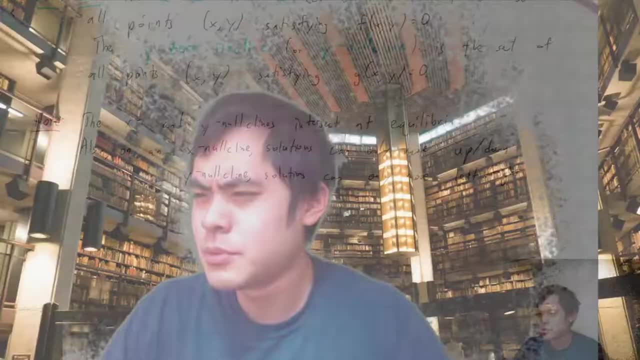 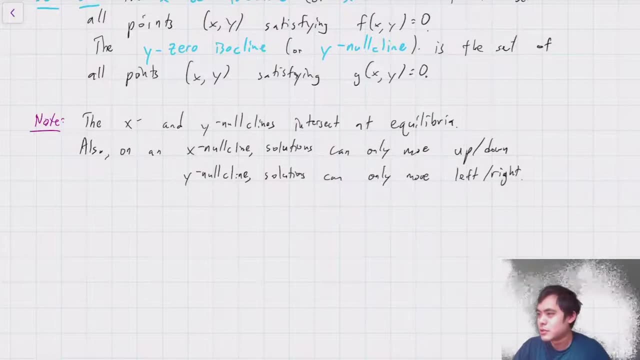 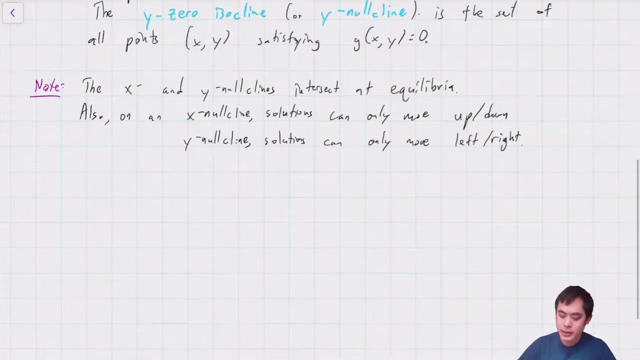 they have a special name of nocline. Just a moment, It looks like my webcam green screen is going all jittery. Oh there, Okay, Okay. So let's get back. Let's actually see an example of this. Just jump straight into examples, since that's a little bit easier to understand what I'm talking about. 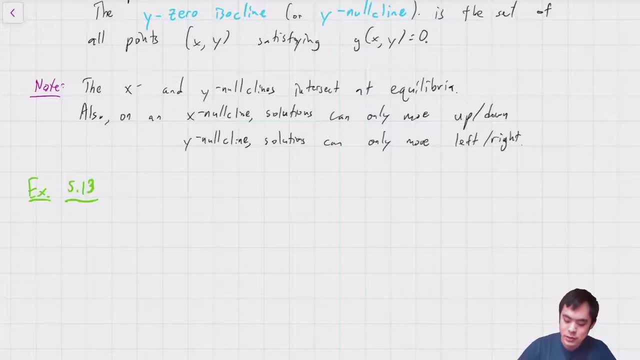 So this is example 5.13 in Linda Allen's textbook. So we have started out with our two equations: dx, dt. Let's say that's equal to xy minus y, which we'll find it useful later to have this in factored form. 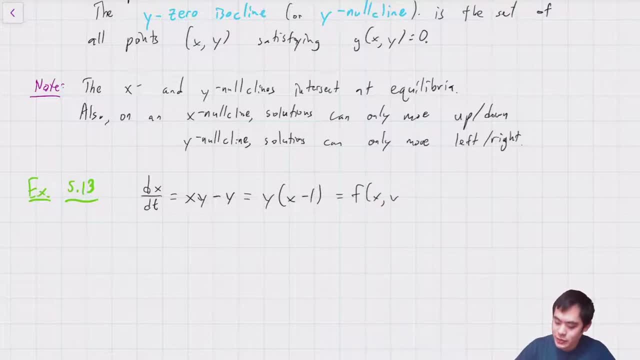 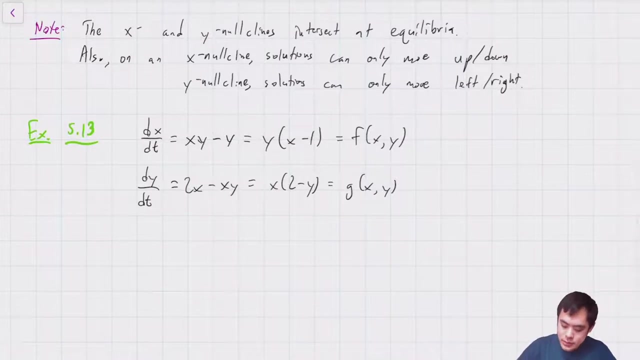 y times x minus 1, which is some function f of xy. And we have dy: dt is equal to 2x minus xy, which is equal to x times 2 minus y, which is equal to some function g of xy. Okay, 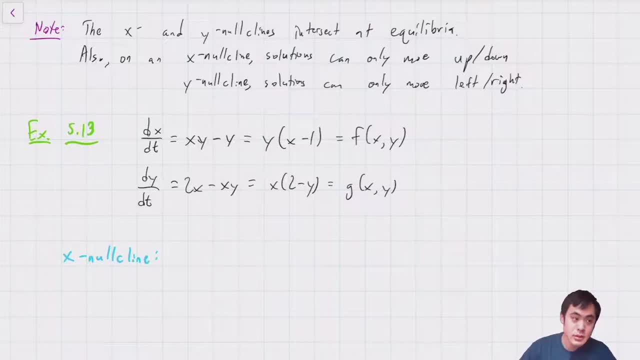 So what's our x nocline? Let's do this in blue. So that's when dx, dt is equal to 0. So 0 is equal to y times x minus 1, which implies that y is equal to 0 or x is equal to 1.. 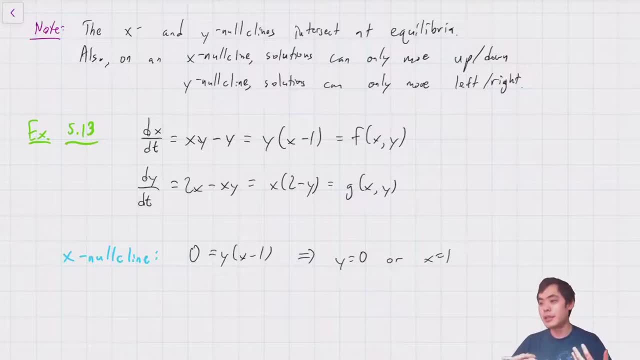 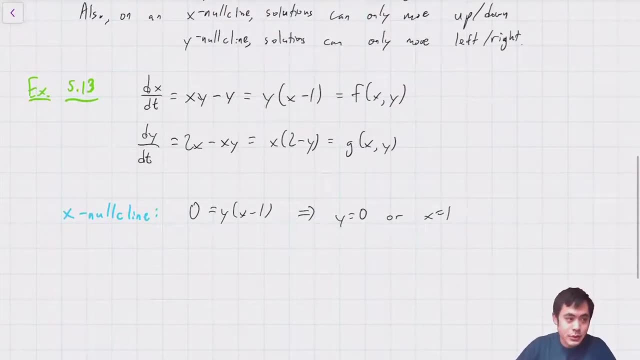 Note that all of this is two different lines. This is all just the nocline, the x nocline, So it's just a single thing Because it's the set of all those points. And we also have the y nocline, which is when 0 is equal to x or times 2 minus y. 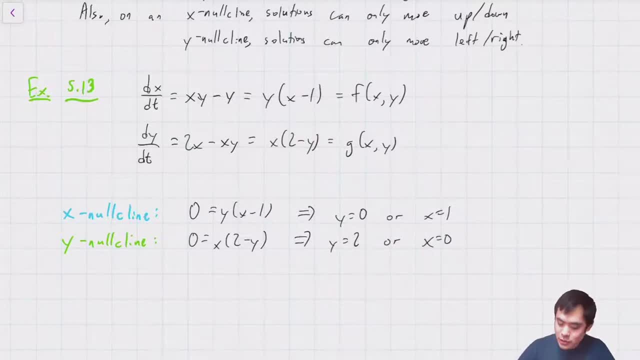 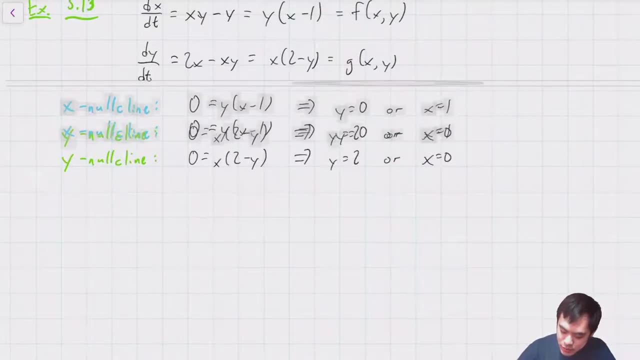 which implies that y is equal to 2 or x is equal to 0.. And let's draw this out. So let's see, Actually, let me move this up, since we don't need all that space, And let's try to fit all this on a single page. 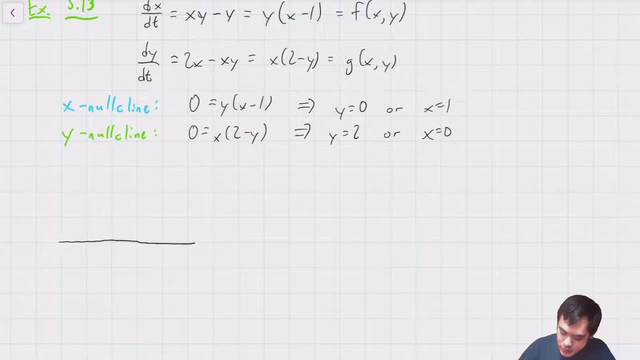 Okay, So we have our x nocline, which is y equals 0.. And let's see, This is the x-axis, This is the y-axis, So y is equal to 0.. So we have that, And we also have when x is equal to 1.. 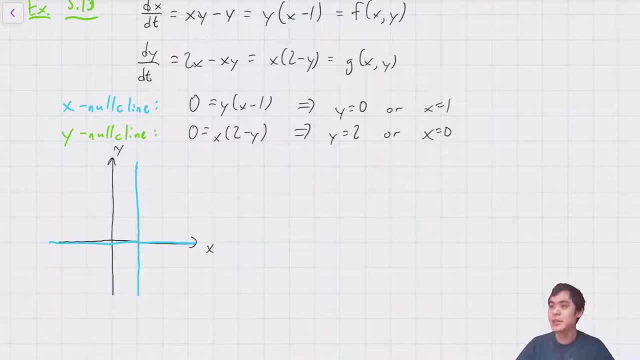 So all of this blue set here is the x nocline And then the y nocline. that's going to be y is equal to 2 or x is equal to 0. So all of that set is the x nocline And one of the things we'll notice. 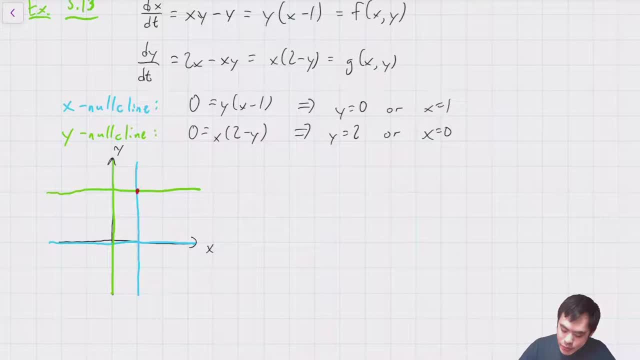 is that when the two intersect you get an equilibrium. So we have our equilibria points here. So equilibria, Or when they're both equal, when both f of x- y and g of x- y equals 0.. 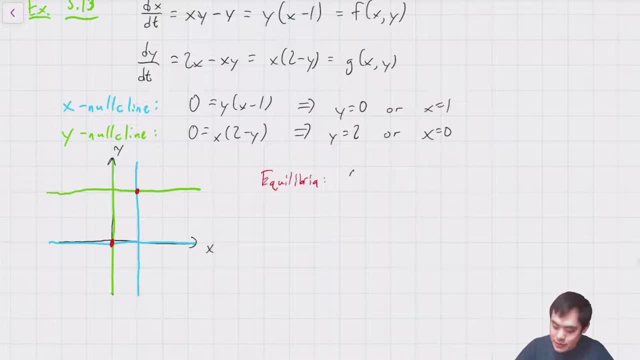 So this is at the intersection points, And so that is precisely 0, 0 and 1, 2.. Note that the point 0, 1.. So this here is not an equilibrium, because it's not the intersection of the x nocline and the y nocline. 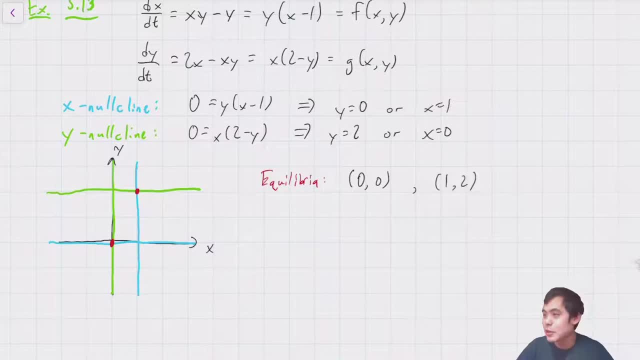 It's just a point on the x nocline, So be a little bit careful about that. These are not lines per se, They're sets And you're looking at the intersection of these sets. Okay, And one of the other fun facts about this: 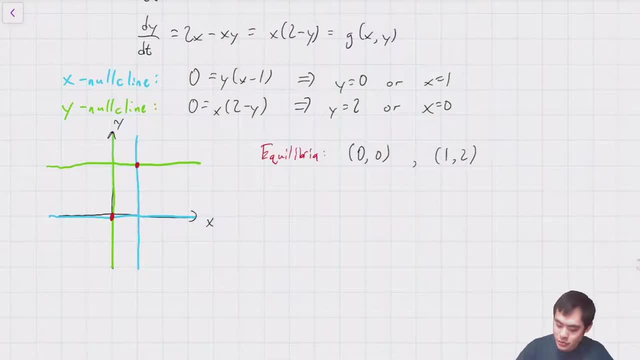 which I am going to ask you to prove in an exercise. So exercise for the viewer is going to be that the arrow direction along a nocline varies continuously, except at an equilibrium, where it'll change direction if the determinant of the Jacobian at the equilibrium 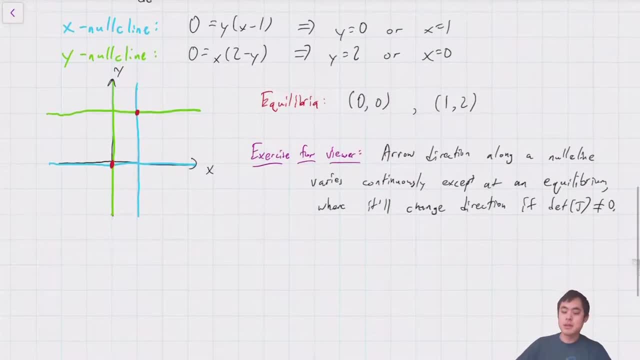 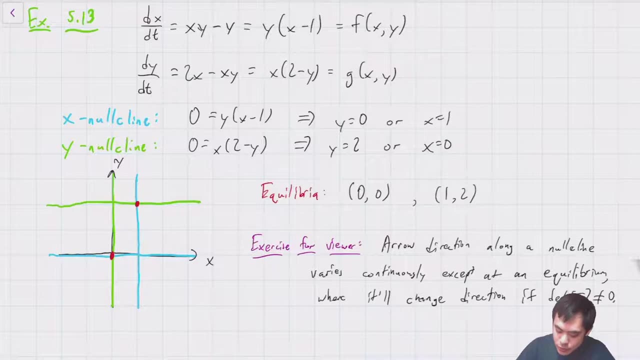 is not equal to 0. What does that mean? Well, we can draw out the vector field, right? So if we have the point here, so let's say we're at the point 1, 1.. So if we're at the point 1, 1,. 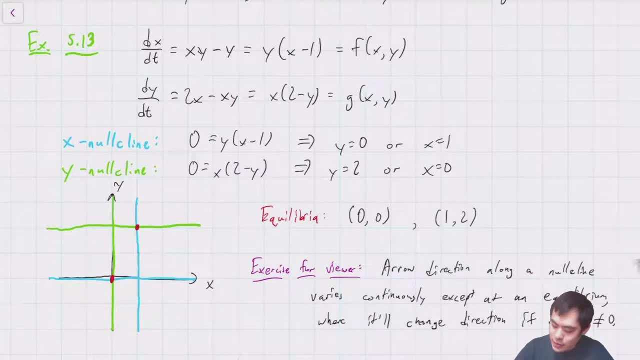 where do we go? So if you plug in 1, so let's see f of 1, 1, well, what's that? equal to f of 1, 1,. you plug in that in, that's equal to 0.. 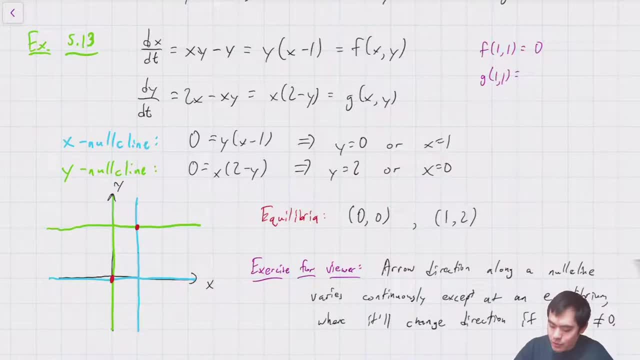 g of 1, 1 is going to be equal to 1 times, so that's 1, right. So that means that here you're going upward in the vector field because you plugged in f of 0, 0 and g of 1, 1.. 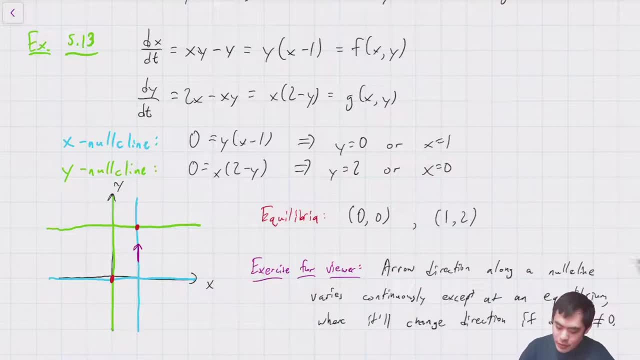 Or sorry, f of 1, 1, g of 1, 1.. What about a couple other points? What about above? So let's say, what about the point here? So that's the point. let's see, that's 1, 3.. 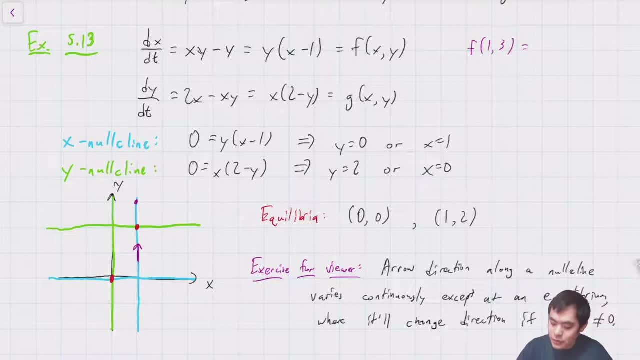 So f of 1, 3.. Well, f of 1, 3, that's equal to 0 again. And this makes sense, right? Because we're on the x-node line, so the f function has to be equal to 0,. 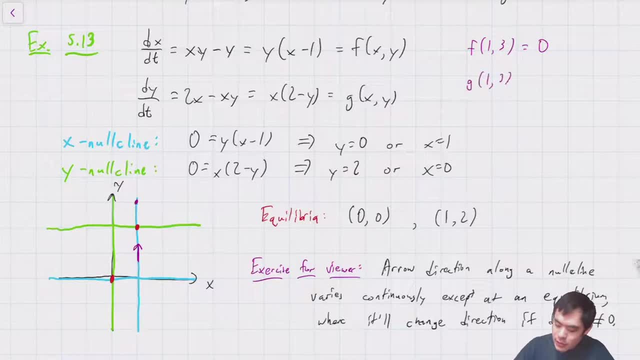 dx, dt has to be equal to 0. And g of 1, 3,. well, that's equal to minus 1.. And so that's going down. What about, at let's say, f of 1, negative 1?? 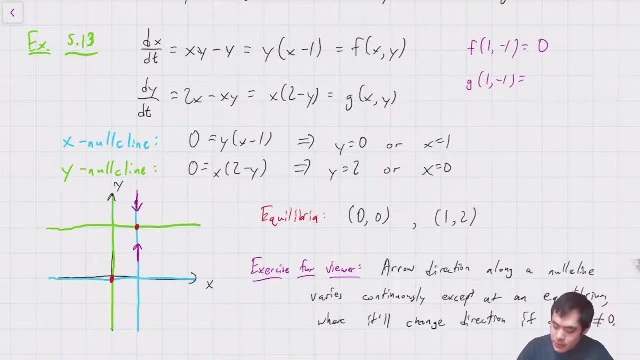 Again, f of 1, negative 1 has to be equal to 0, because we're on the x-node line. And minus 1, let's plug in minus 1 there- that's equal to 3. And so this is also going up. 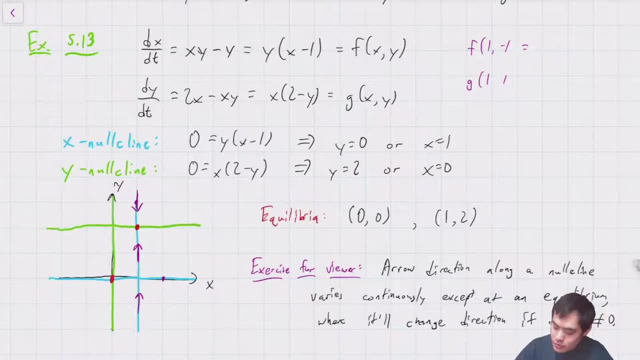 What about at the point 2, 0?? So at the point 2, 0,? well, that is still on the x-node line, so that value is still equal to 0.. So the x-direction value is equal to 0. 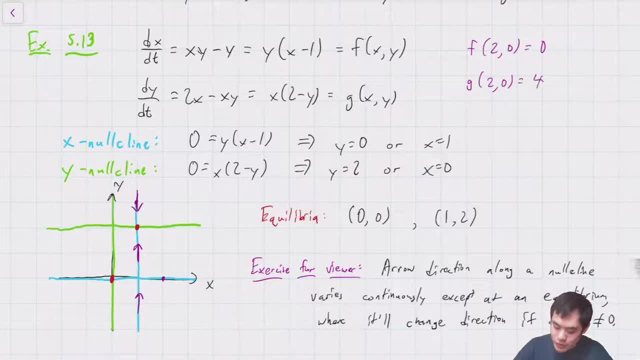 But g of 2, 0 is equal to 4. So that is still going up, because that's the y-coordinate That's going up. And it turns out that if you look here that's also going up. But if you look at the point here, 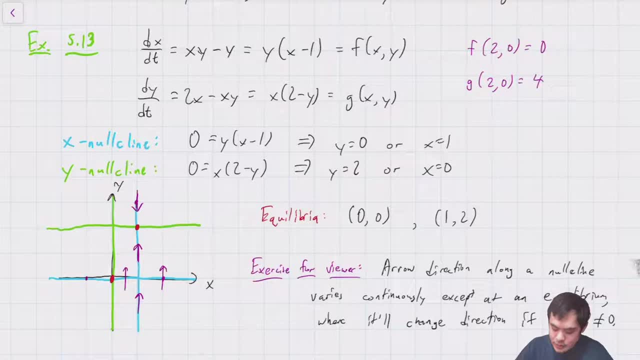 so that's what Minus 1, 0.. So g of minus 1, 0.. Well, f of minus 1, 0 is still equal to 0,, but g of minus 1, 0, well, what does that equal to now? 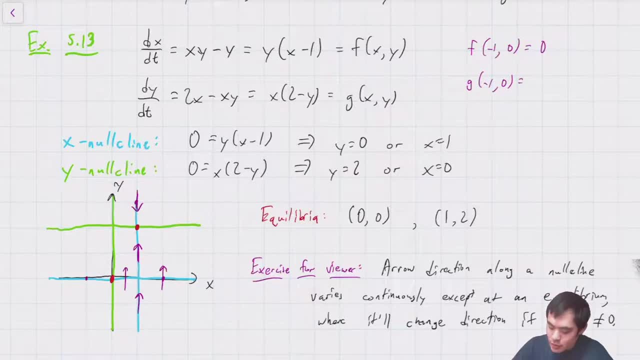 g of minus 1, 0,, so that's equal to minus 1 times 2,, so that's minus 2.. So now we're going down, And you can also check that this one also goes down. And so, as you see, 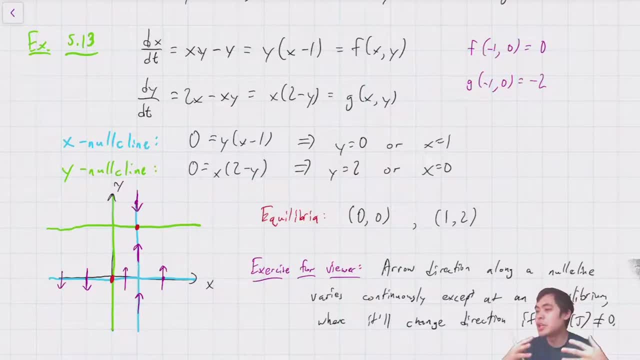 so as you're moving along one of your little node lines, it only changes arrow direction along one of your at the equilibria. And it won't always change direction on an equilibrium, but it sometimes will. Let's do the same thing along the y-node lines. 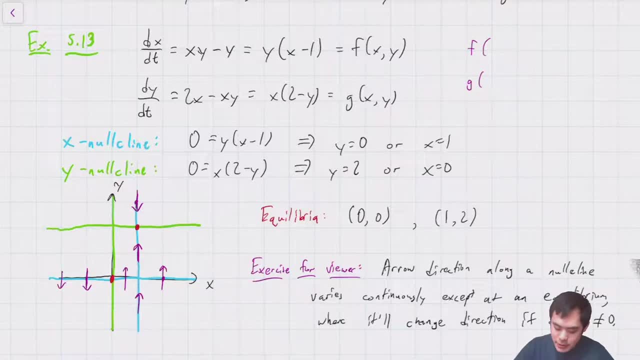 Let's look at a couple of different points. So let's say we're going to look at f of minus 1, 2.. So that's this point up here: minus 1, 2.. Well, here the first thing to notice. 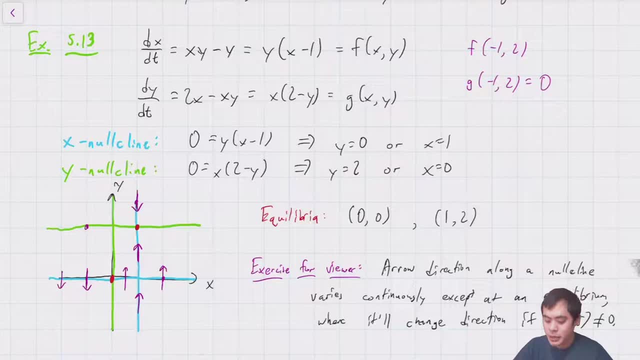 is that dy, dt? so the g function is going to be equal to 0, because you're on the y-node line, Whereas f of minus 1, 0 is going to be equal to 4.. So that is going in the 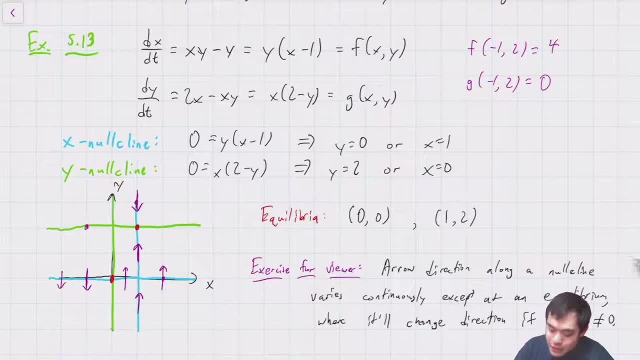 wait, did I do that right, Minus 1, 2.. Oh, I did that wrong, Yep. So minus 1, 2, so that's 2 times minus 1, minus 1,, which is equal to. 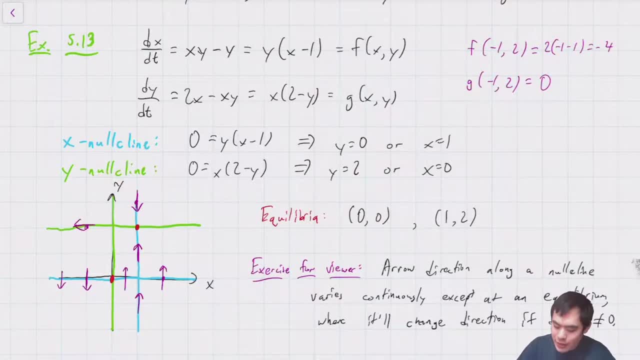 equal to minus 4.. So this is going in the left direction And if we look up here, so let's have 3, 0.. So if we look at 3, 0,, well, it's still on the y-node plane. 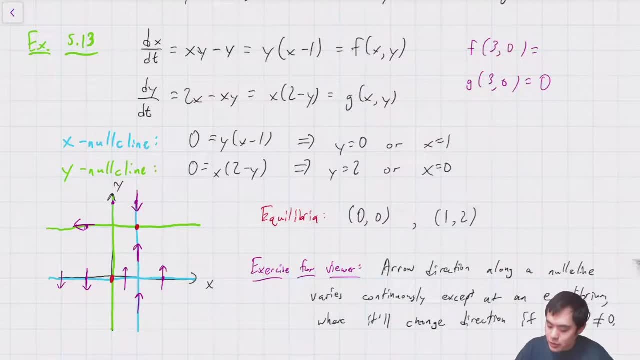 so that's going to be equal to 0.. But 3, 0 here. well, that's going to be equal to wait a moment. what did I do wrong? Oh sorry, 0, 3.. Not 3, 0.. 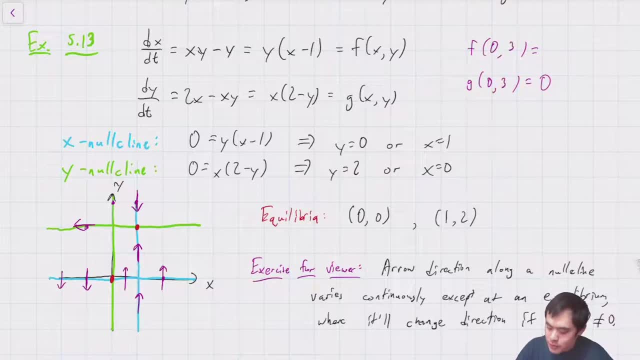 0, 3.. So that's that point up here. 0, 3, that's going to be equal to minus 3 and 0. So it's going along the x-axis, it's going in the negative direction. 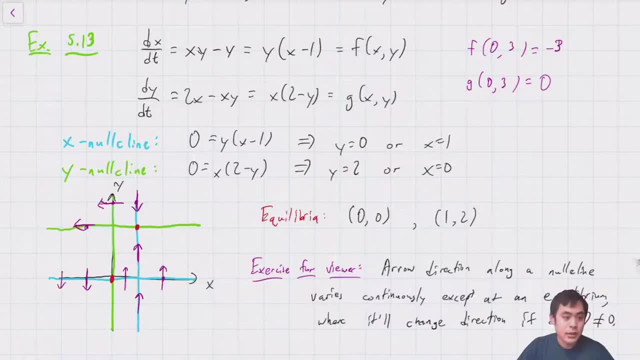 so that's still going this way And with a little bit of checking you'll find that it goes this way there, this way here. so it goes in the positive direction there and over here it switches direction and again and goes to the right. 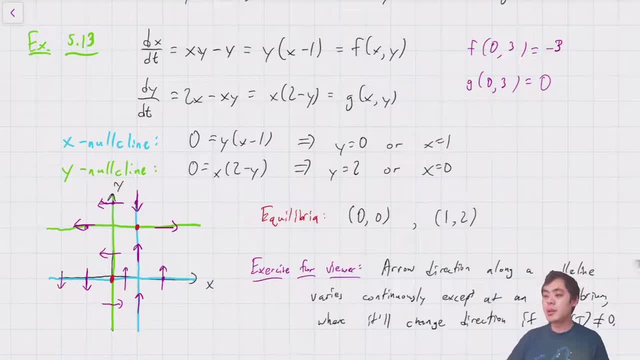 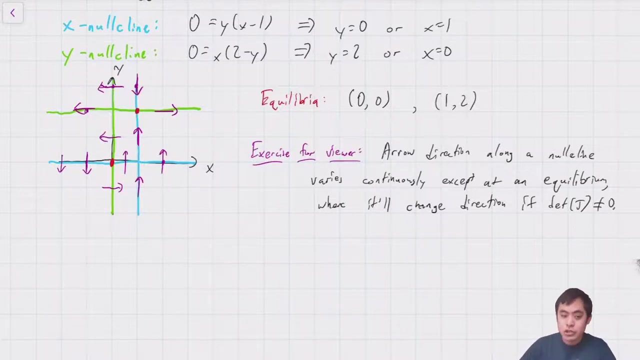 And so this gives us some sense of where these directories go. So it gives you a partial vector field and you can follow along. So one of the things that we should have checked, actually- which would have made this a lot easier- is if we knew the Jacobian. 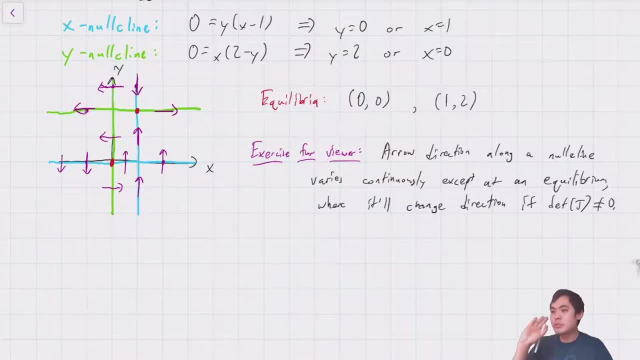 of the equilibria, we would know whether or not it switches direction when you cross it. Here, empirically, we've seen that. oh well, it does seem to switch direction when you cross the equilibria, And so, therefore, the equilibria. 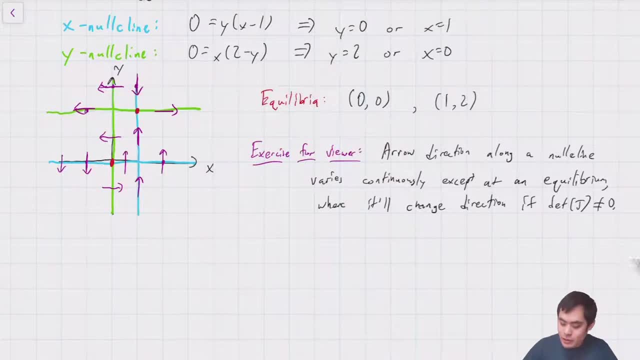 probably have the term that's not equal to zero. I mean, well, they definitely have it, but let's go ahead and verify that. So j of x- y, the Jacobian matrix is just going to be y, x minus one. 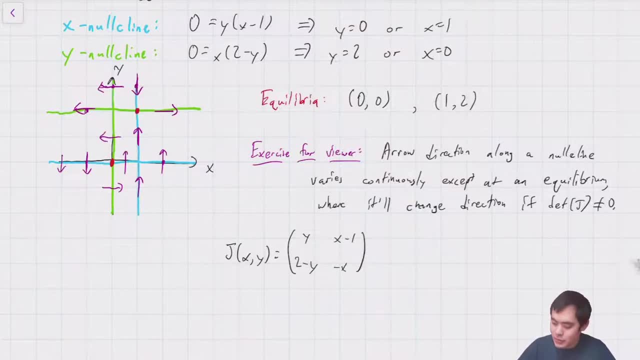 two minus y and minus x. That's something pretty easy to verify. So j of zero zero is going to be equal to zero minus one two zero, And j of one two is going to be equal to two zero, zero minus one. 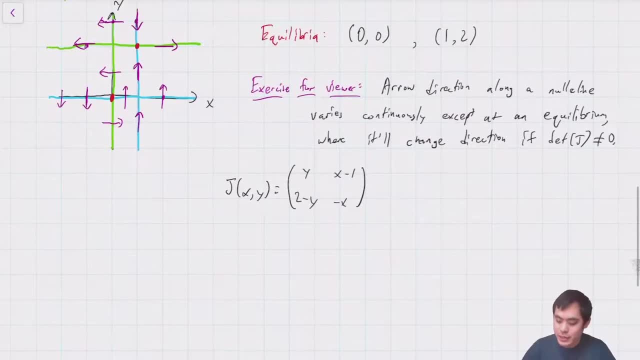 Let me actually write this out in a little bit more space, since we're going to be doing some additional analysis on this in a moment. So j of zero zero is going to be equal to zero minus one two. zero j of one two. 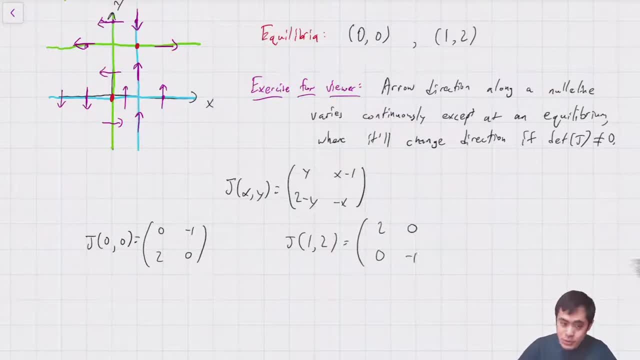 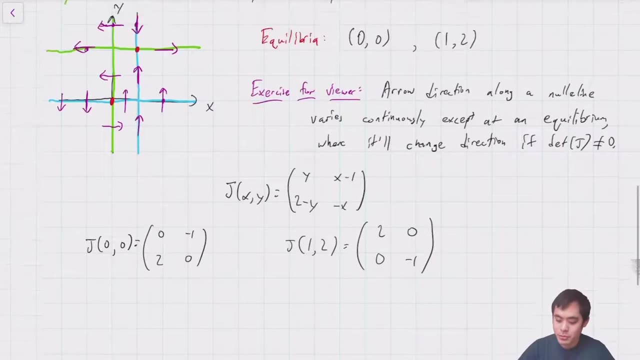 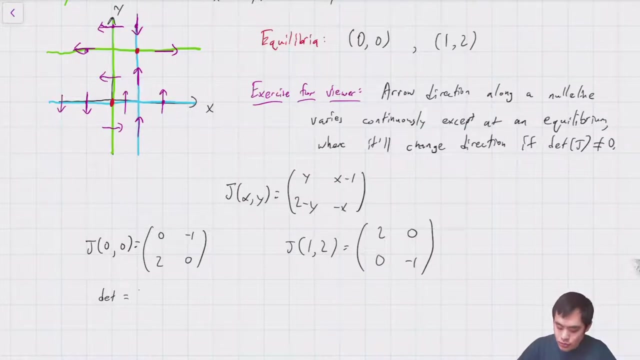 is going to be equal to two, zero, zero minus one. And so we can compute, explicitly, compute the eigenvalues and find the determinants of Euler, please. So the determinant here is going to be equal to well, it's going to be equal to two. 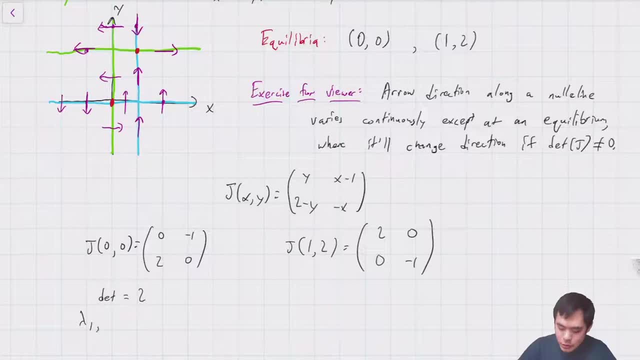 And lambda one is going to be equal. lambda one and two are going to be equal to plus or minus. i times the square root of two And the trace here is equal to zero. Here the determinant is equal to minus two. Trace is equal to one. 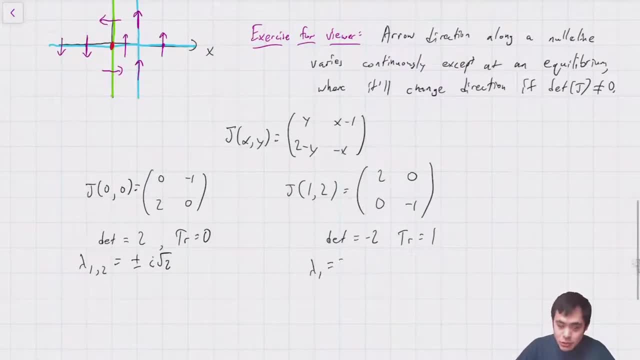 And we have two eigenvalues: Lambda one is equal to two and lambda two is equal to minus one. So we could also compute the eigenvectors. It's pretty easy in this case: One zero and zero one, And so one of the things 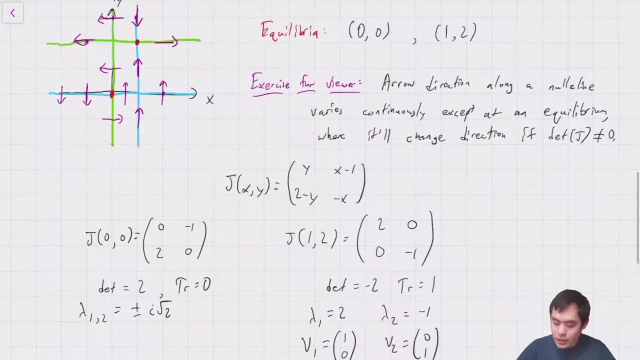 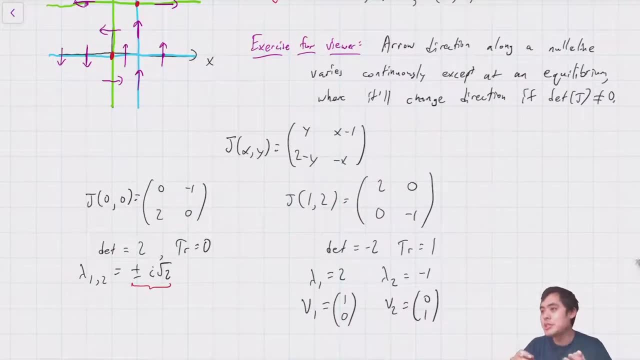 you can do is you can look locally around each of these things and see what's going on. So here this thing. here we think is, if this were linear, this would be a center. We don't necessarily know this for certain. There are other tools. 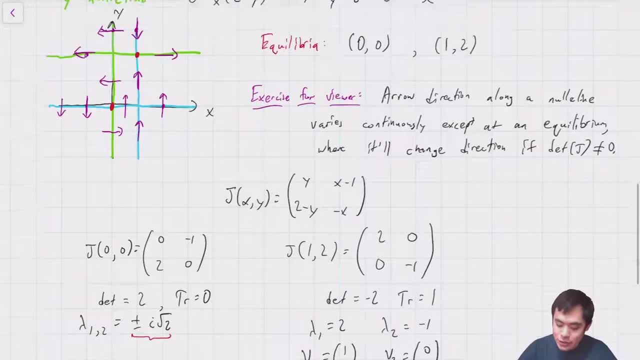 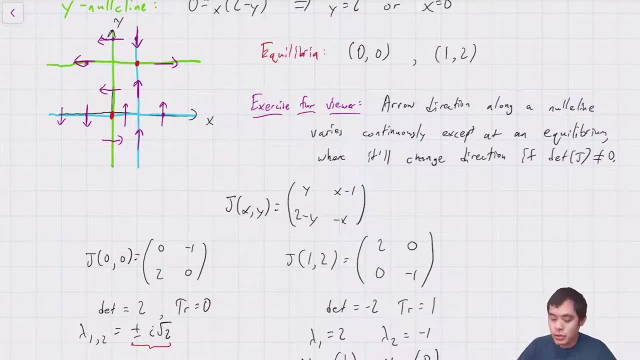 we can use to show this. And it does turn out that it is a center in this particular case, And if you draw some trajectories, what you're doing is you'll note that the trajectories have to be tangent to your vector field, And so you end up. 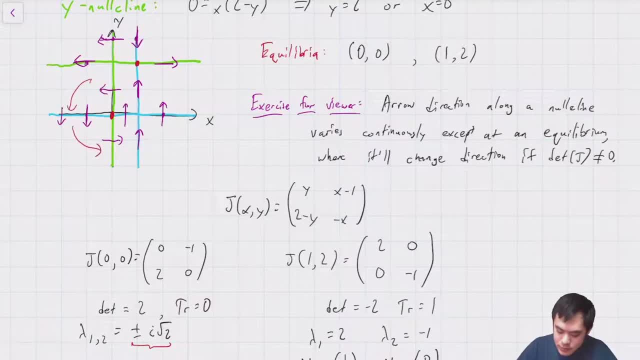 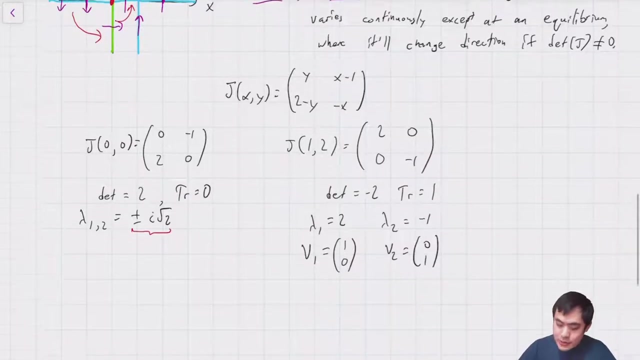 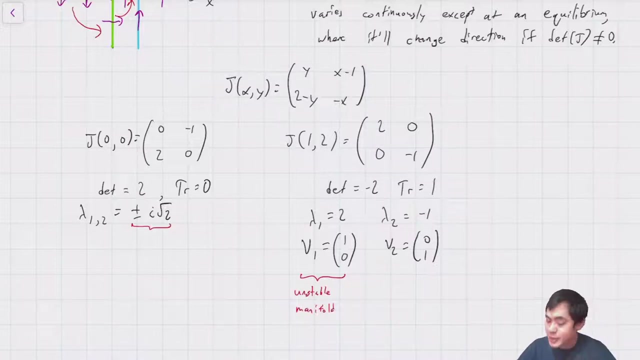 with things like this And so on, And one of the things you can do is locally around this equilibrium. So that's this equilibrium. down here We have the unstable manifold and the stable manifold. So this is called the unstable manifold Because the eigenvalue 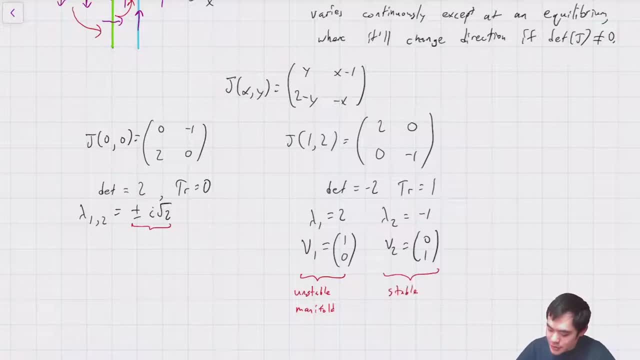 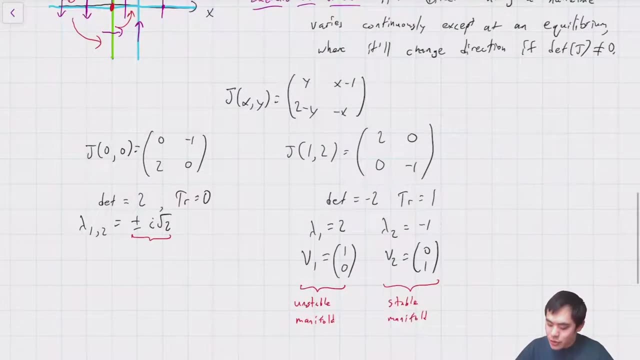 is positive, And this is the stable manifold. Note that this is the saddle point And that's what unstable and stable manifolds are defined for. And so along the x-axis, so in the horizontal direction, things are going out, And in the vertical direction, 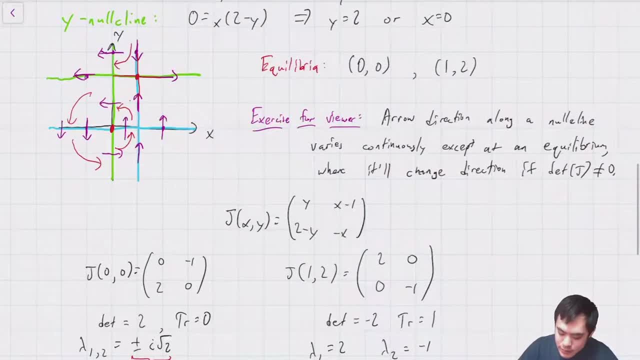 things are going in. So you end up with things like that. And if you draw a couple more trajectories, you might end up with something like this And note that the directions- because the directions along- note that when you're crossing the manifold, 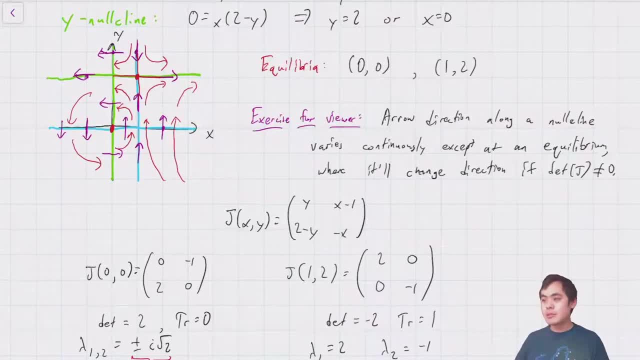 when you're crossing the isoclines, you have to cross it orthogonally to the isoclines, Or sorry, not orthogonally. You have to cross it either in the up direction or in the left or right direction. 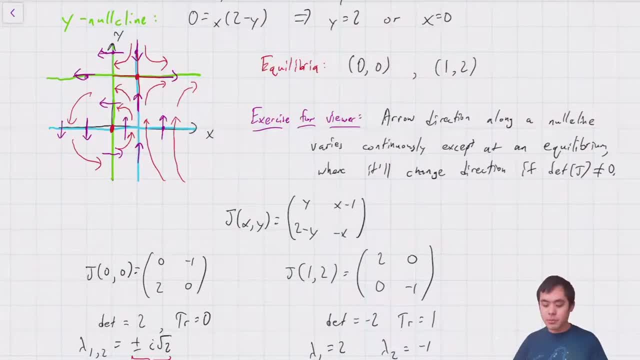 depending on if it's the x or y isocline Which allows you to say more things about the function in general. So this is our handwritten drawing based on this isocline analysis of this phase portrait. We can also do this by looking on. 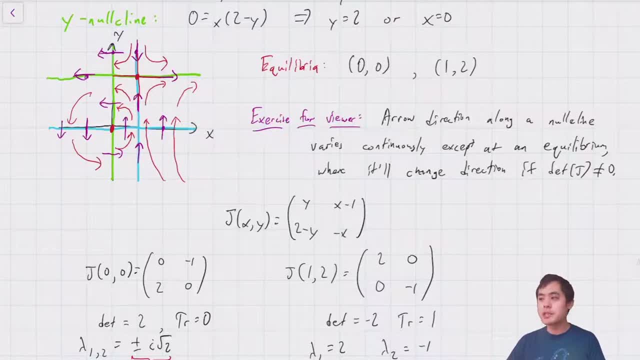 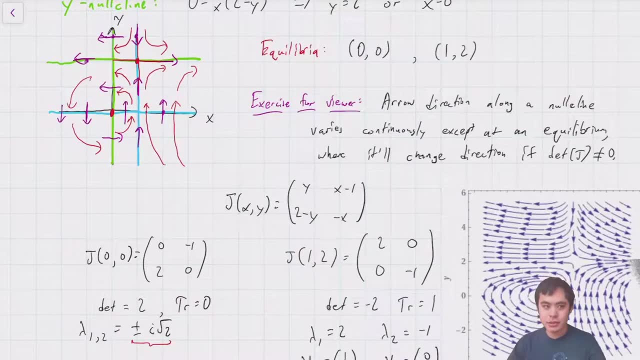 having a computer draw out the phase portraits and trajectories, And when we do we'll see that this is actually pretty close. So I took a moment and, off camera, I went on Wolfram Alpha and had to draw a stream plot of this particular graph. 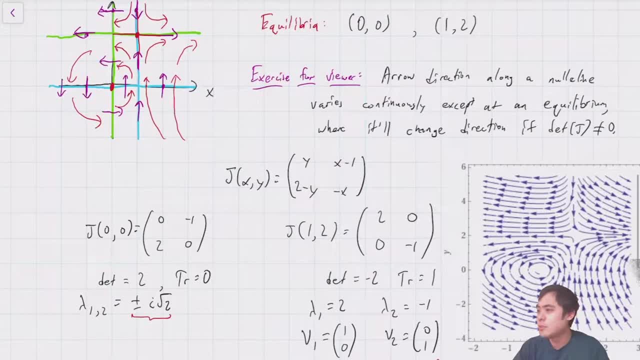 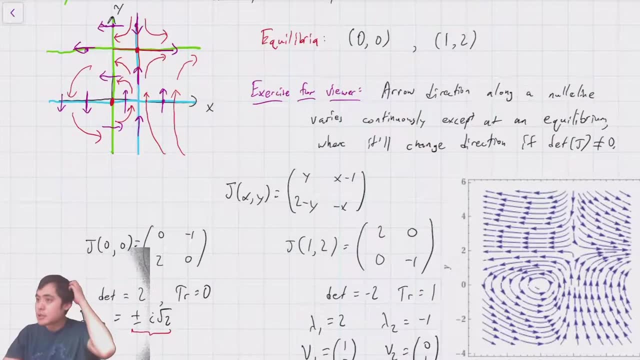 so that you could see the similarities between the two. Actually, let me move myself out of the way so that this comparison is a little bit easier. So, as you can see, the stream plot, the trajectories that we drew over here, are pretty similar.